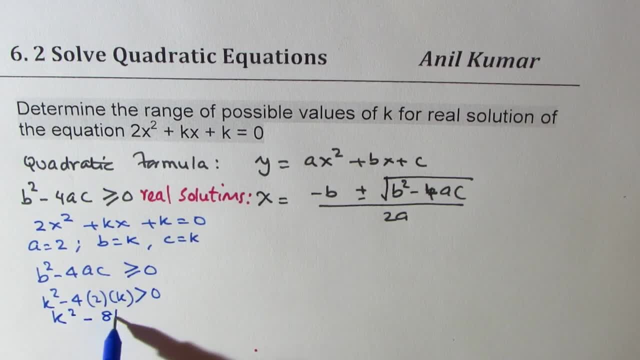 So what we get here is k square minus 8k should be greater than or equal to 0 for real solutions, correct? Now let us see how to solve this inequality. So what we could do is we could factor k out. 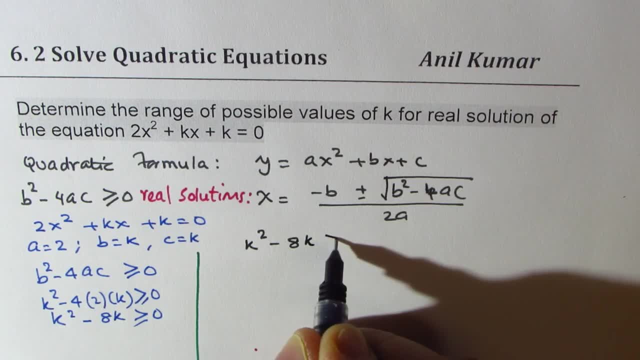 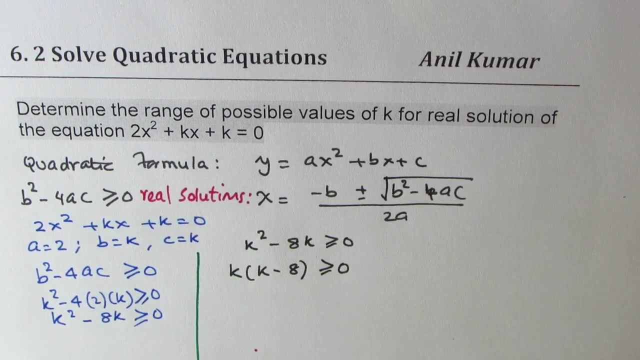 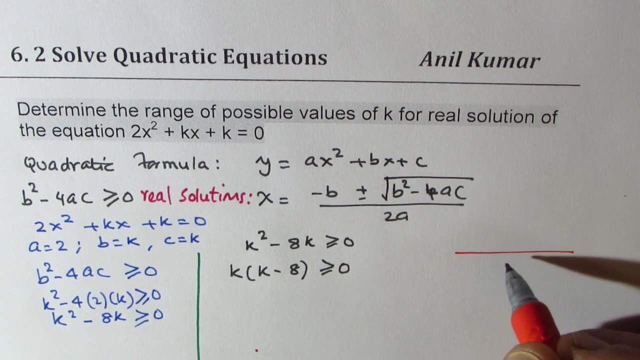 So we have here k square minus 8k greater than or equal to 0. If I factor k, I get k minus 8 greater than or equal to 0.. Now you could do it using table of values. You could also do it sketching a graph, correct. 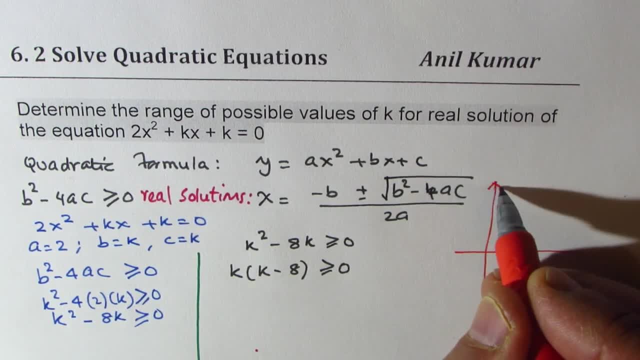 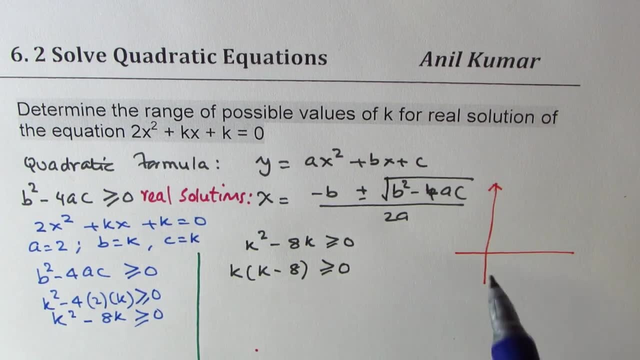 So we have two 0s, one at 0,, the other one at k, equals to 8, right? So, and this is a parabola which opens upwards, This is at 0,, the other one is at 8.. 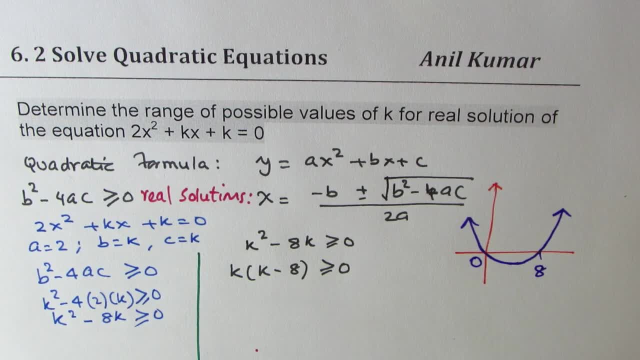 So we have to see when is it greater than or equal to 0.. So we have to see when is it greater than or equal to 0.. So from this graph it is very clear that the solution is either towards the left side of 0 or right side of a correct. 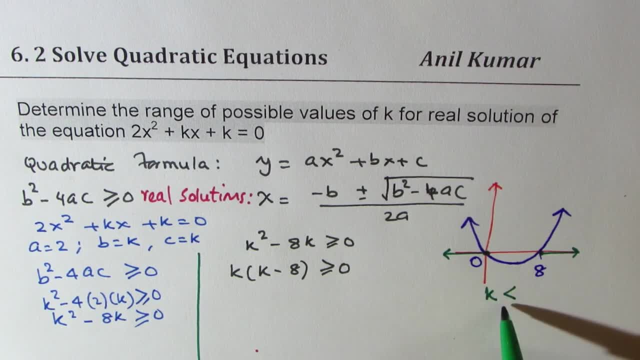 So we have the value of k, that it could be less than or equal to 0, or k should be greater than or equal to 8.. So that becomes our solution. This is one way of doing it. Now we do have another way of solving this question. 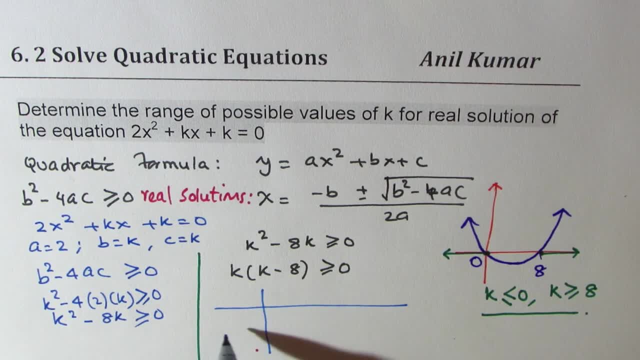 And that is to. So we have two 0s here. One is at 0.. So the graph could change the value at this 0 and also at the other right, So we can take test points in these intervals. 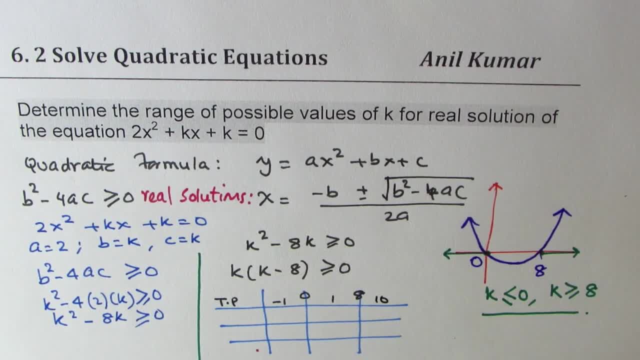 A test point: minus 1, here we could take 1, and here we could take 10.. So for k, if I substitute minus 1, it will be negative. If I substitute 1, it is positive 1. 10 gives me positive 1.. 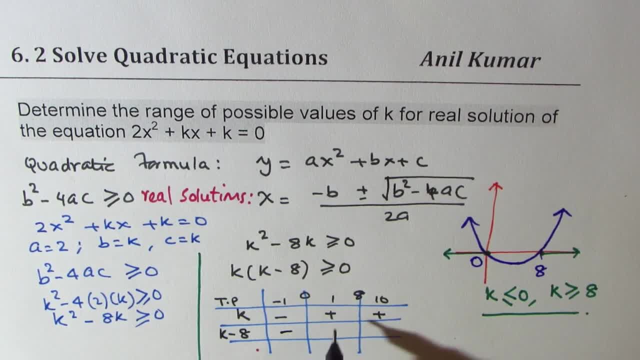 For k minus 8, this will result into negative. That will also give me negative, And here I'll get positive. So what we get here is that these two negatives, when multiplied, gives me positive. Here we get negative.